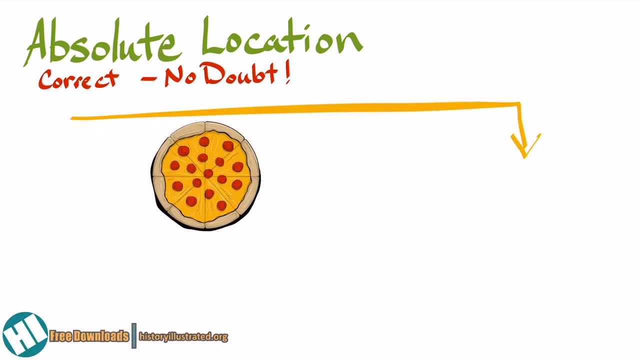 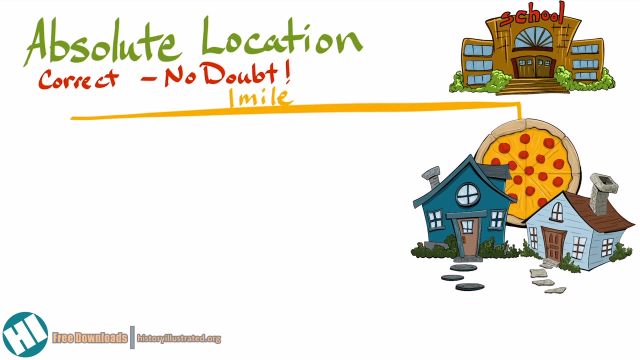 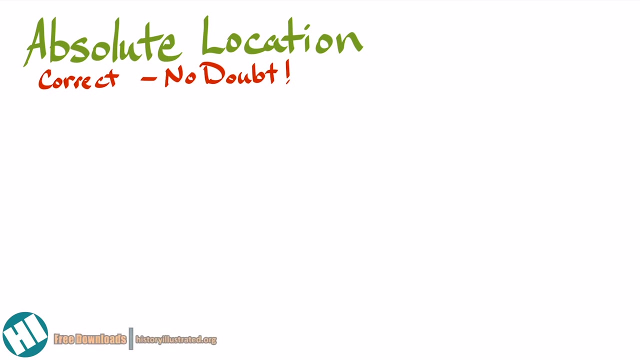 Like my house is one mile down the road. on the right, It's the blue house across the street from the school. This works well most of the time. But what if there are two blue houses or the driver goes a little under a mile? Maybe they missed the school? Well, an absolute location could work. 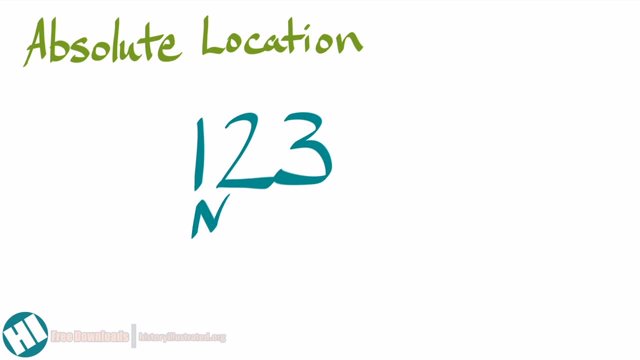 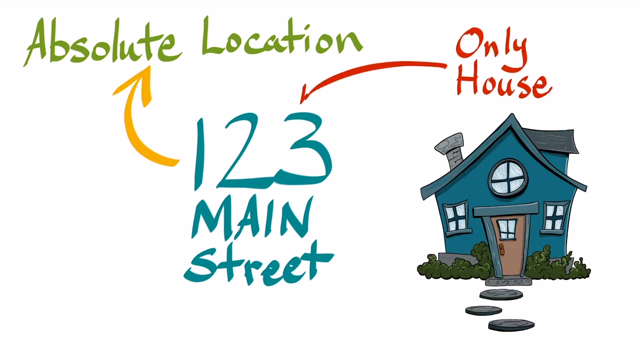 better You could give them the address. Like I live at 123 Main Street. This address is an absolute location. With it I can find your absolute location. I know exactly where you are, Which means this is the only house with this address, so there should be no confusion. 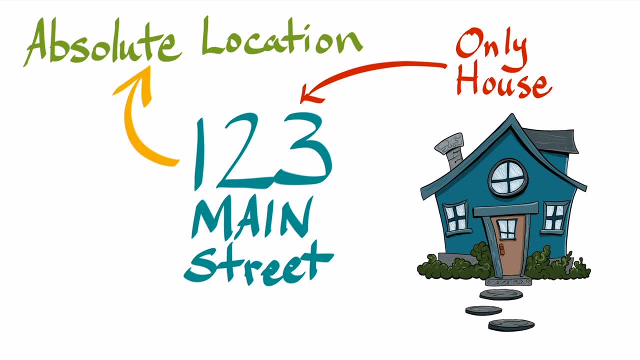 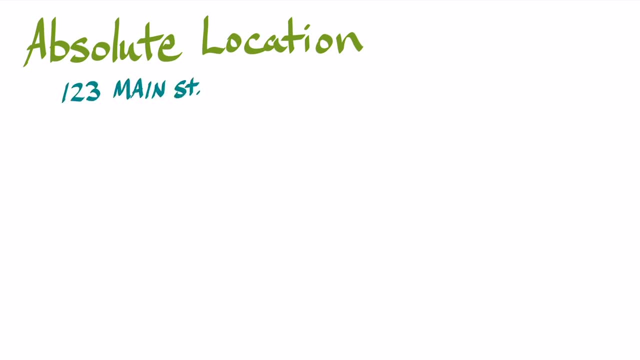 Of course, we do use absolute locations when ordering pizza all of the time, But we might also add some relative locations too, just to make it a little bit easier. Like I live at 123 Main Street- It's the blue house across the street from the school, about one mile down the road. 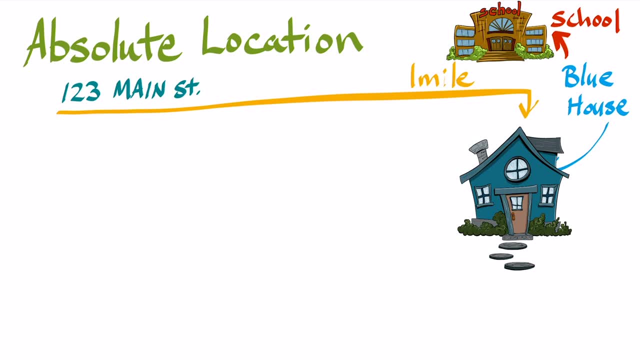 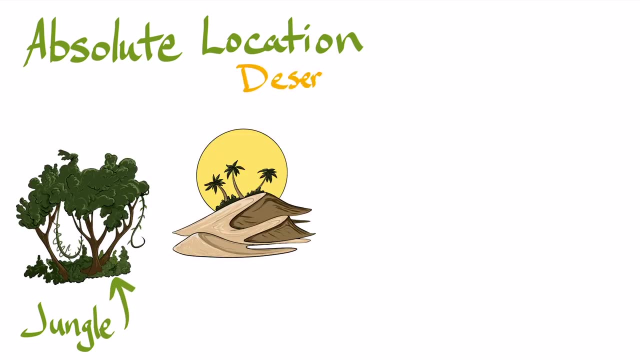 Combining them makes it easy to find the locations most of the time. Sometimes addresses don't work, though. What if you're in the middle of the jungle? What's your address? What about the desert, The Arctic? Or what about in the middle of the ocean? Is there an? 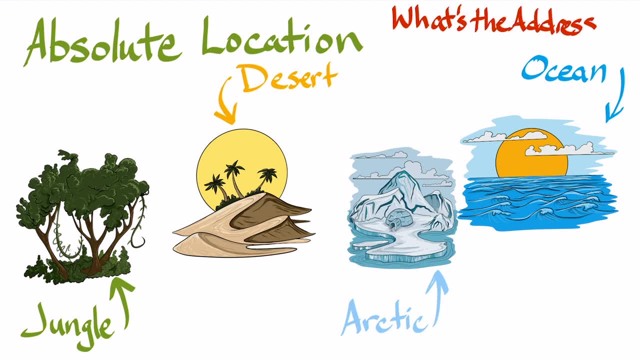 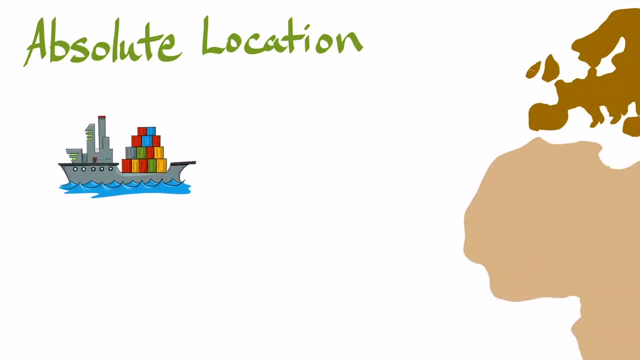 address for that. Well, this is a good time when we can switch over to use coordinates, Which we discussed in another video. For example, a boat is trying to find its way to the Canary Islands off the coast of Africa. The boat is 30 degrees north and 15 degrees west. By looking at those, 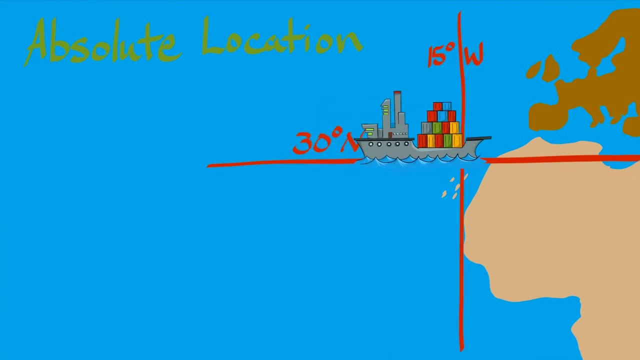 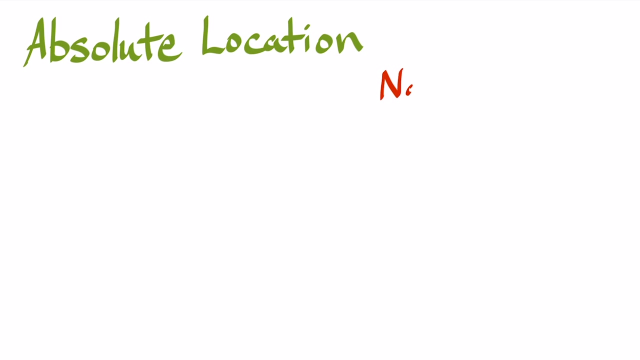 coordinates. you can see the boat is close, but it's not quite there. Giving the exact coordinates of the Canary Islands can get you to where you're going. This is an absolute location. You could also give them relative location directions and tell them that they are north. 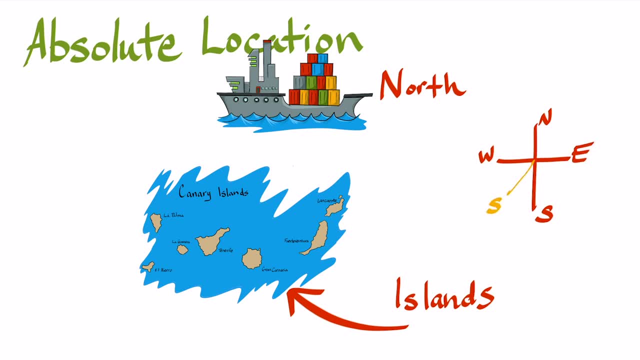 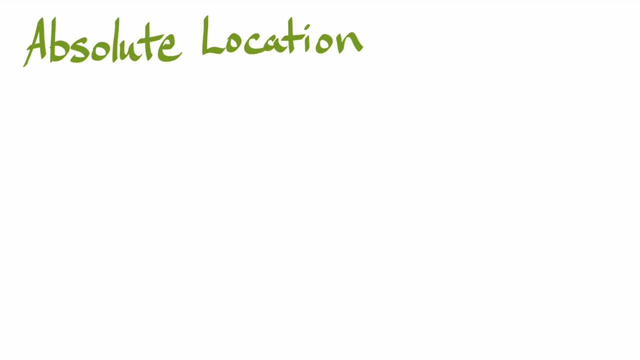 of the islands and they need to sail south- southwest from their current location. Both of them could help out, But the coordinates are precise. There is no need to describe what they are looking for. In conclusion, absolute location uses man-made systems like coordinates or addresses. 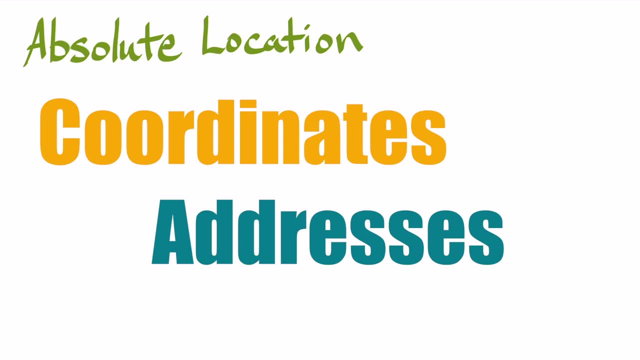 A precise location of something in order to guarantee there is no confusion in finding it.